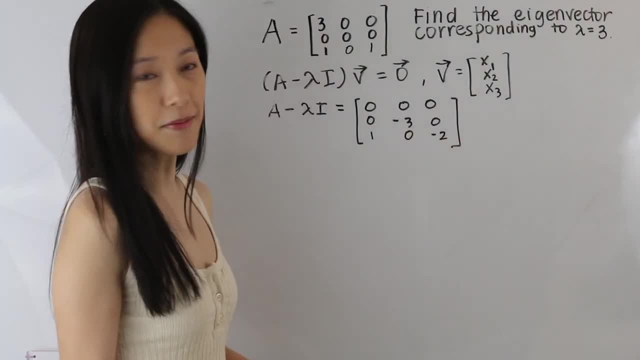 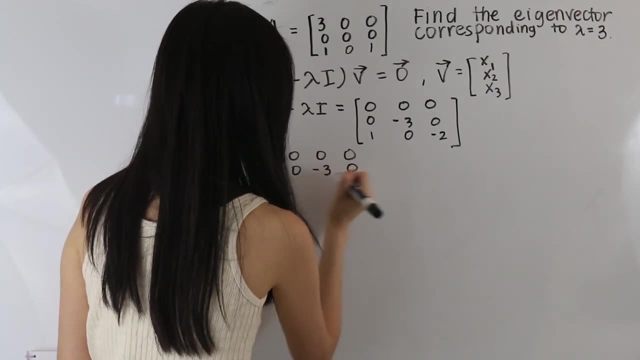 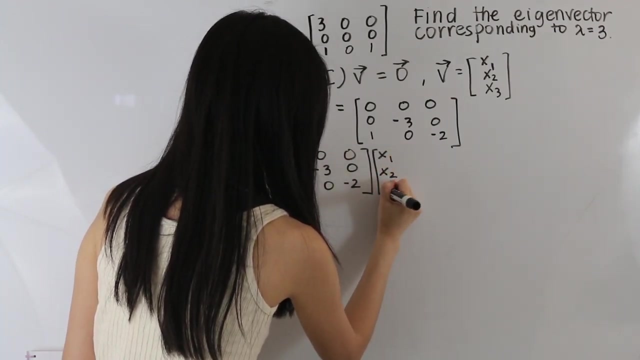 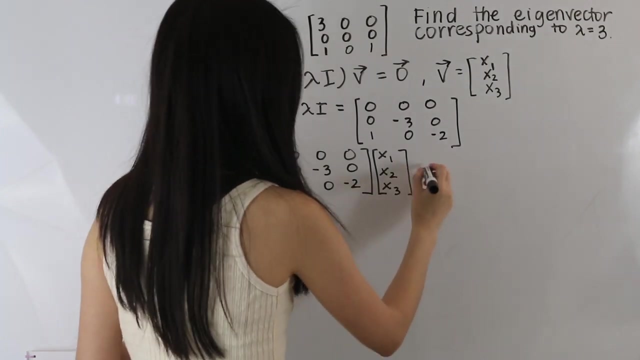 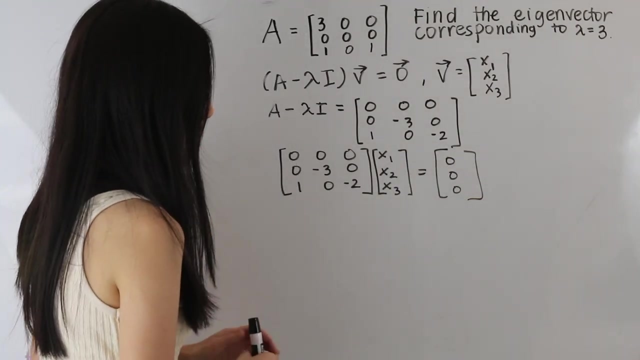 So the next step is we're going to plug this into here, And V is just the eigenvector. we were solving for this, And then this is equal to the following: The eigenvector, So just the zero vector, And so we can rewrite this in the form. 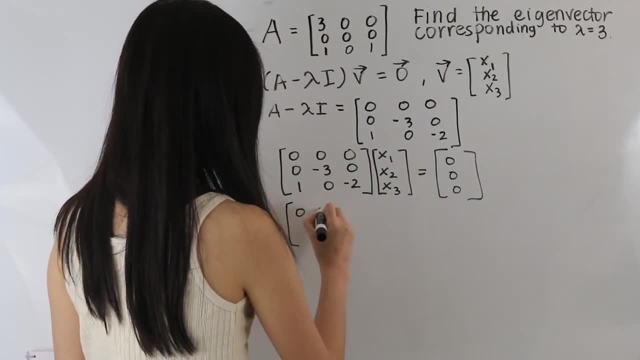 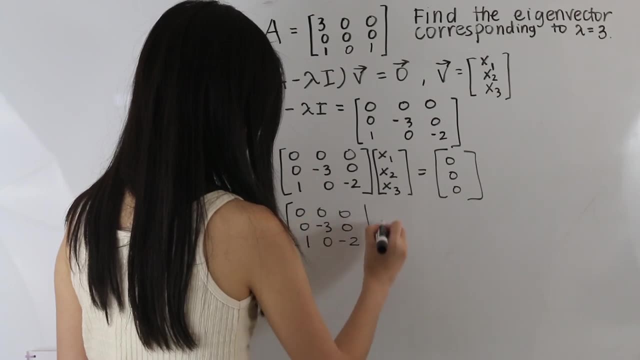 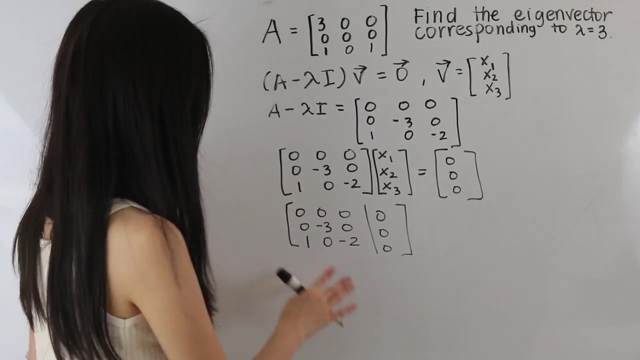 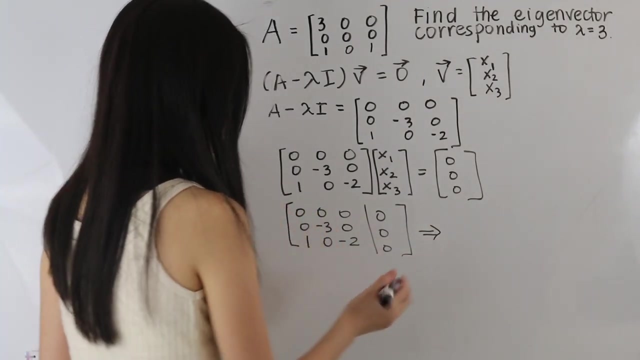 of an augmented matrix. So that's gonna look like this, And so from here we're gonna want to use row operations to get this into row echelon form. So first let's start off by interchanging the first row and the third row. 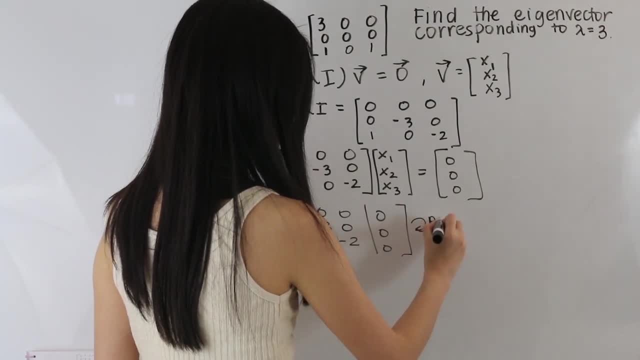 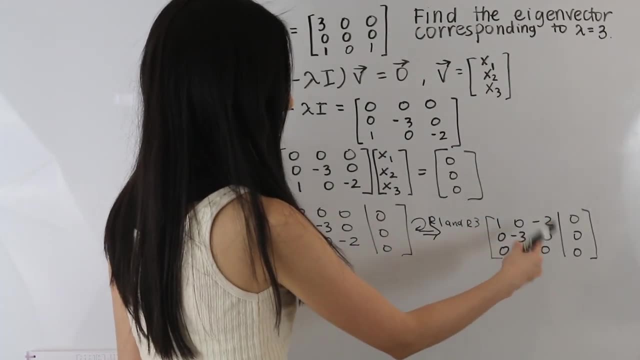 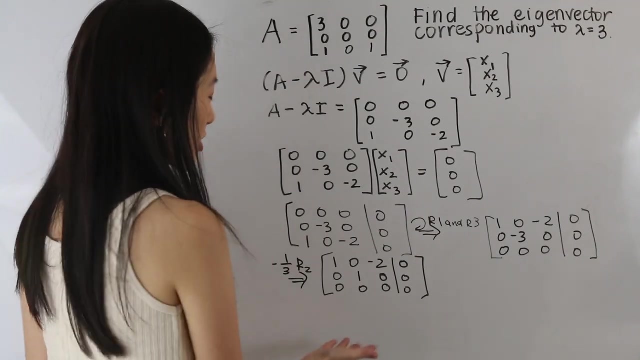 So let's go ahead and do that. So the next thing that we're gonna want to do is turn this negative three into a one, So we're gonna multiply row two by negative 1. 1. 3rd, And so now we have our matrix in row echelon form. 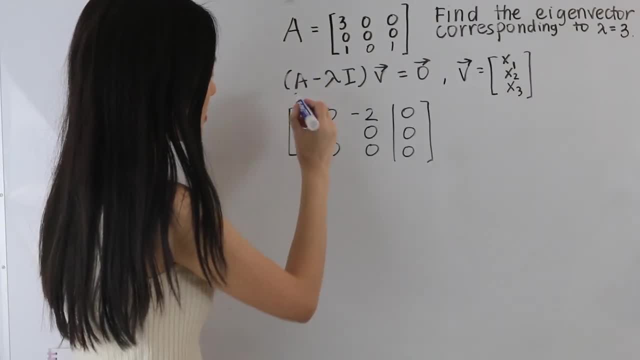 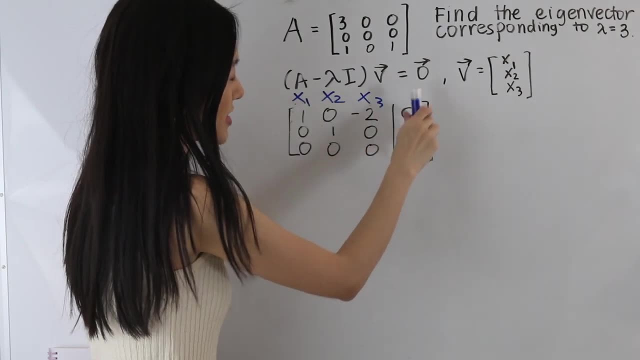 So, just to note, this column corresponds to X1, this column corresponds to X2, and this column corresponds to X3.. And this is just. this is just one column corresponding to this vector here, And so let's go ahead and circle our pivots. 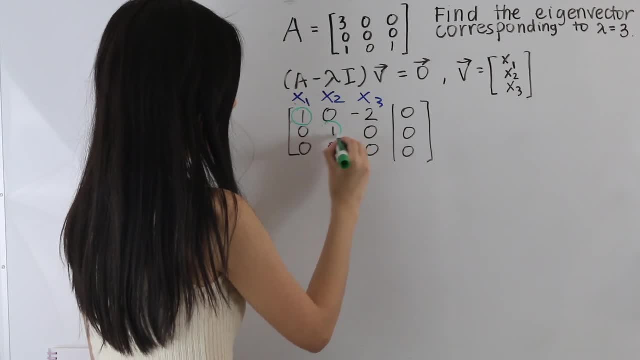 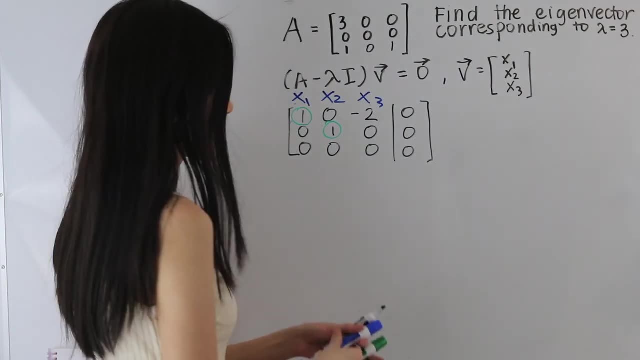 So we have this one here and this one here, And the reason for this is because any column that does not correspond to a pivot is considered a free variable. So here, because X3 does not correspond to a pivot, X3 is considered a free variable. 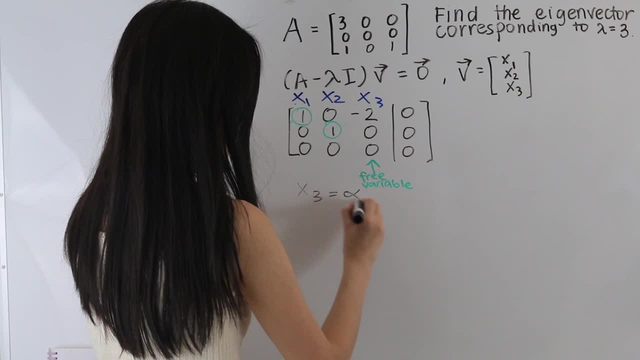 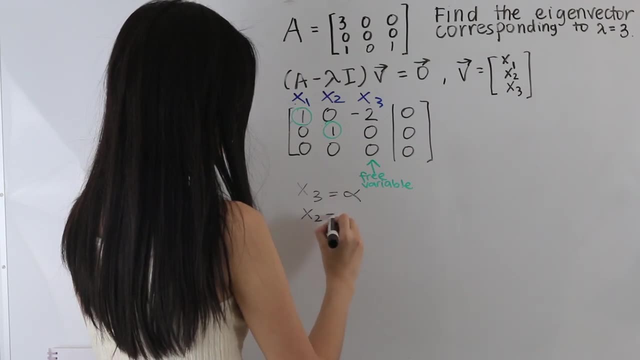 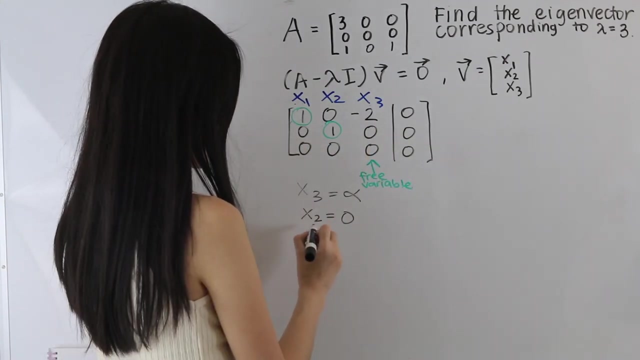 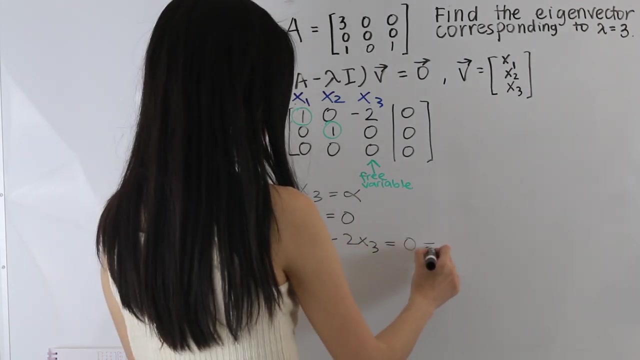 So we can set X3 to alpha And then next from this row here we have: X2 is equal to zero, And from this row right here we have: X1 minus 2X3 is equal to zero, And we can rewrite this as follows: 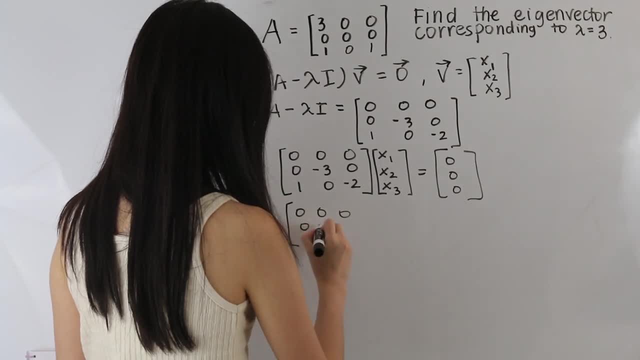 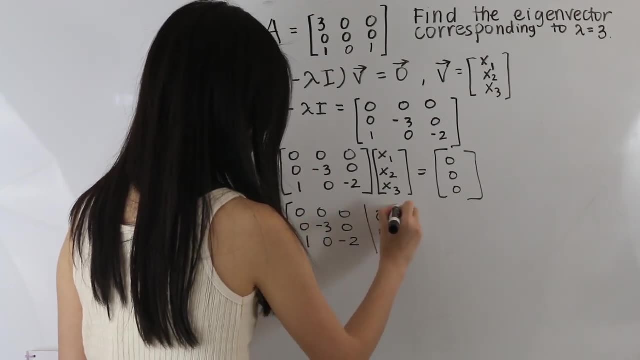 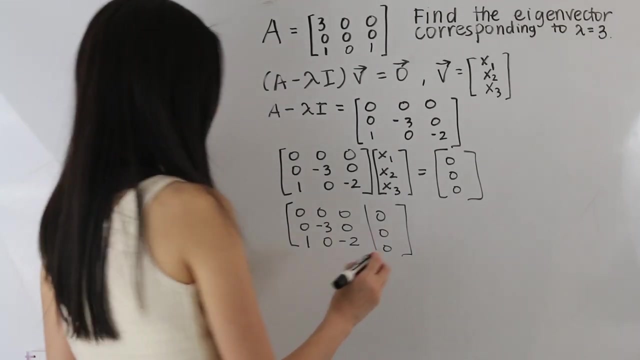 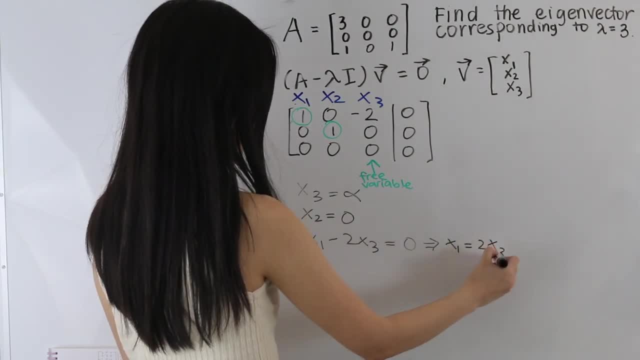 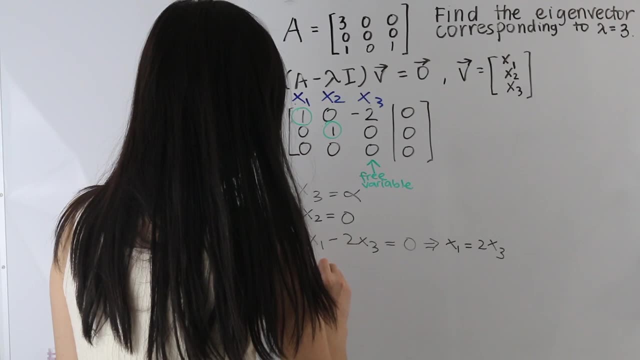 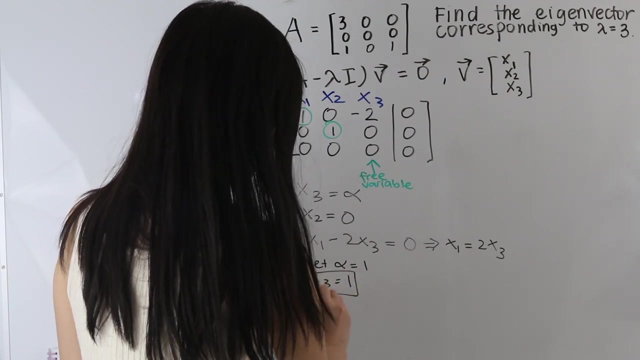 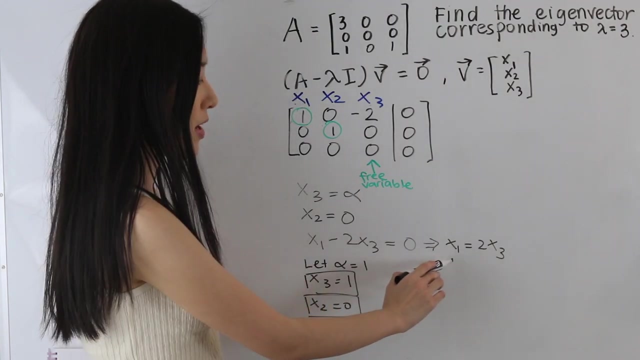 So we have: X1 is equal to 2X3.. So let's go ahead and let our alpha equal to one, So we get X3 is equal to one, And we have X2 equal to zero, And we have X1 equal to 2X3. 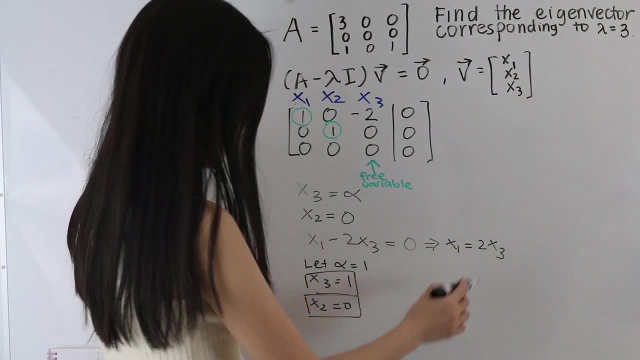 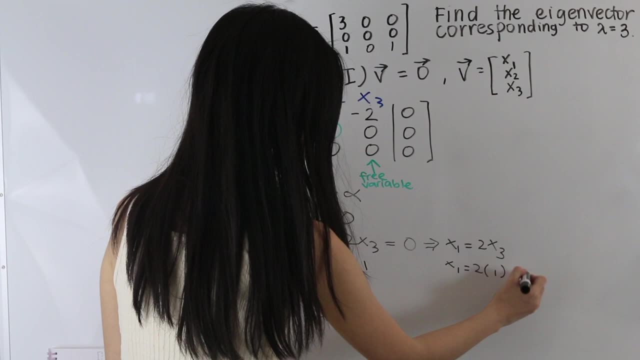 So let's go ahead and plug in our value for X3 into here. So that gives us X1 is equal to 2X3,, which is just two times one, which is two. So we have X1 is equal to two. 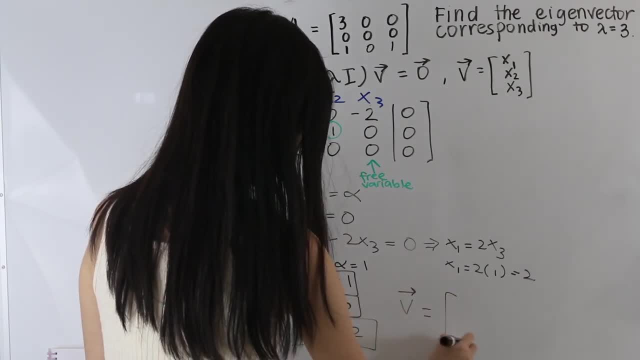 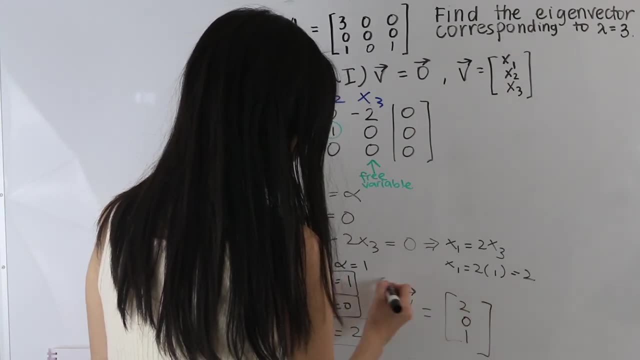 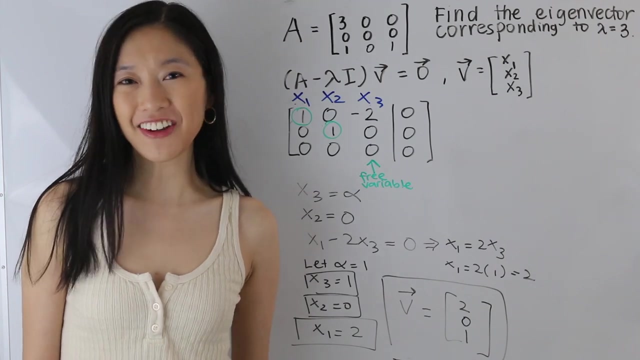 So we have our eigenvector: X1 is two, X2 is equal to zero, We have X3 equal to one. So that is our eigenvector, And that is how you find the eigenvector corresponding to an eigenvalue of a three by three matrix. 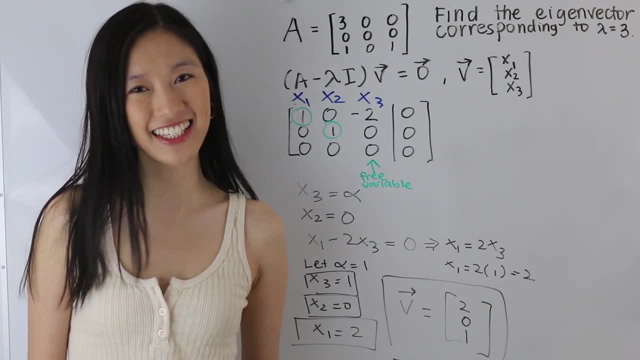 Thank you guys so much for watching. Don't forget to like, comment and subscribe And I'll see you guys in the next one. Bye. 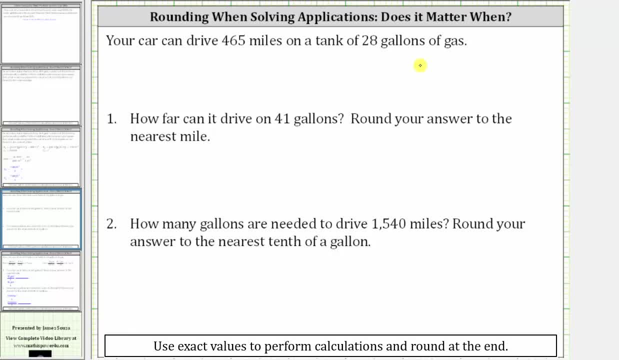 In this video we will look at an example that we are asked to round and we'll show how, when we're asked to round, we should use exact values to perform calculations and then round to the very end. If we round too early, we have much more of an error. 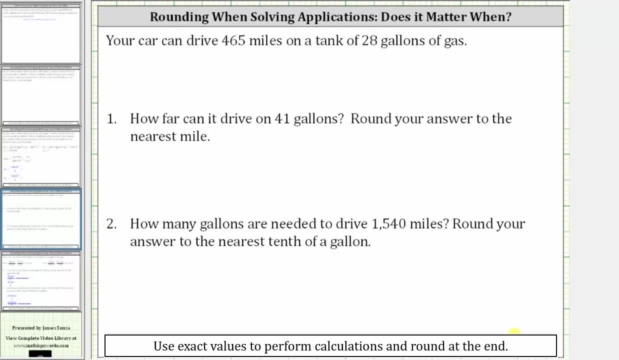 which we should always try to avoid. For this problem, your car can drive 465 miles on a tank of 28 gallons of gas. Number one: how far can it drive on 41 gallons Round? the answer to the nearest mile. Number two: how many gallons are needed? 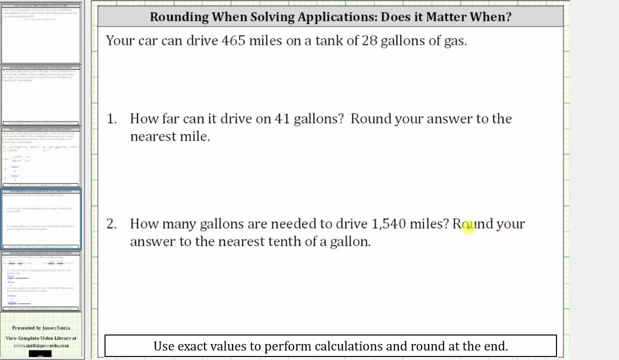 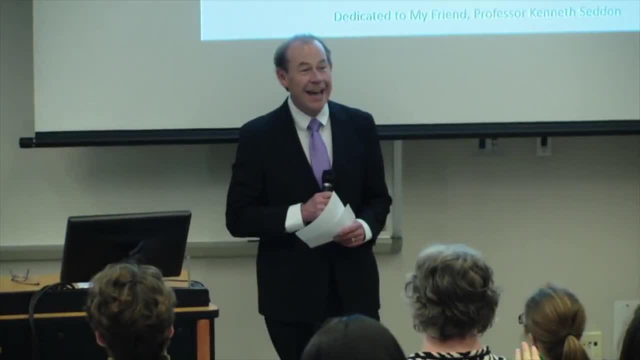 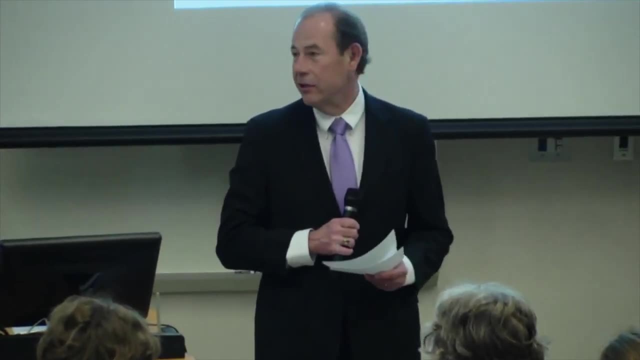 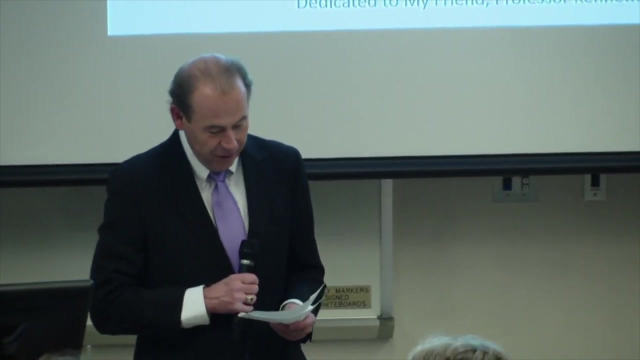 My name is John Sutherland, I am the Fasenfeld Head of Environmental and Ecological Engineering and I would like to welcome you all to the inaugural College of Engineering Distinguished Lecturer. At this point, I would like to introduce Meng Chang, who is in turn going to introduce. 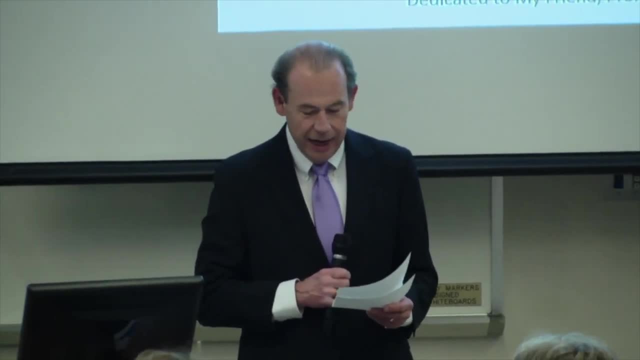 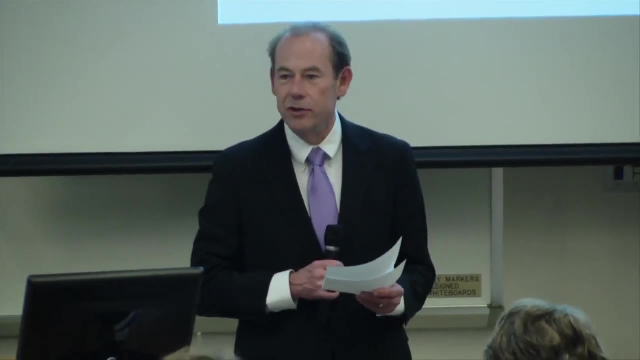 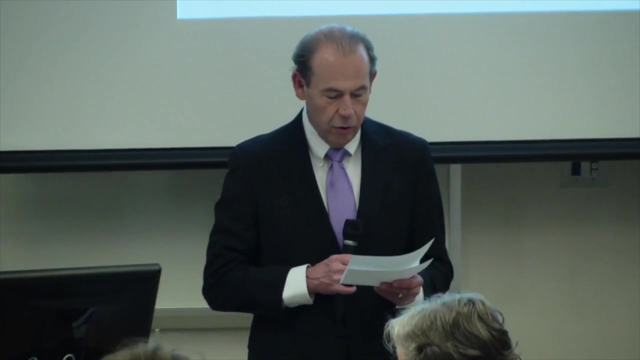 our speaker for today, Dr Chang, is the John A Edwardson Dean of the College of Engineering and the Roscoe H George Professor of Electrical and Computer Engineering. The Dean has impacted over 250,000 students via his courses and textbooks, has co-founded several start-ups. 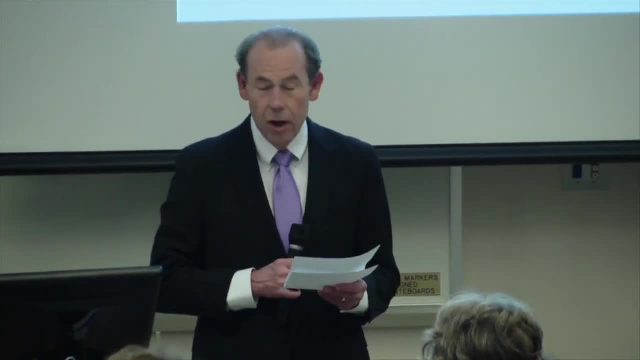 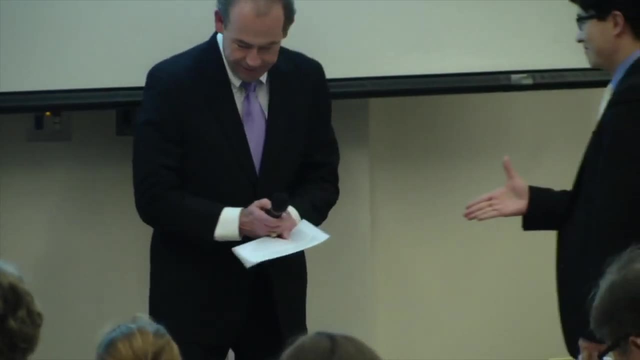 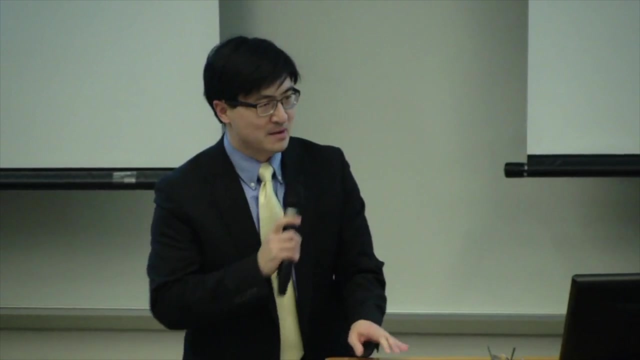 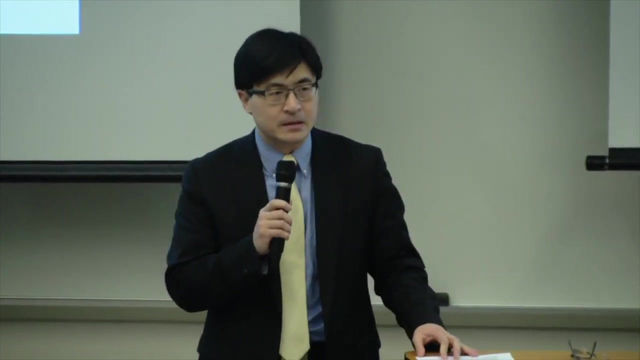 and a non-profit consortium and is also a recipient of the prestigious NSF Waterman Award, Dean Chang. Thank you, John. Good afternoon everyone. Welcome to the inaugural Purdue Engineering Distinguished Lecture Series. Today is the day that we start this series and we have been planning this.